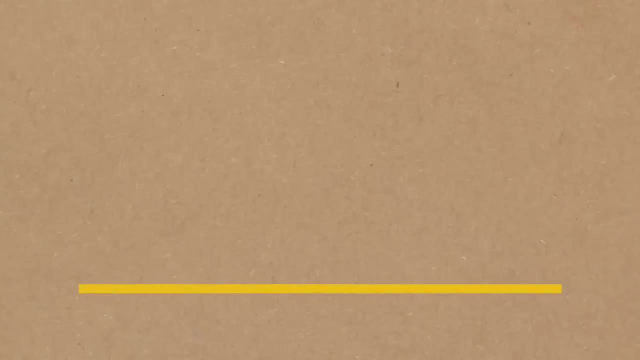 And this time I'm going to ask you a probability question. I'd like you to answer this question on the scale of impossible, ie probability zero up to certain, And I don't really care about a number. If you can give me a number, I'd be impressed. 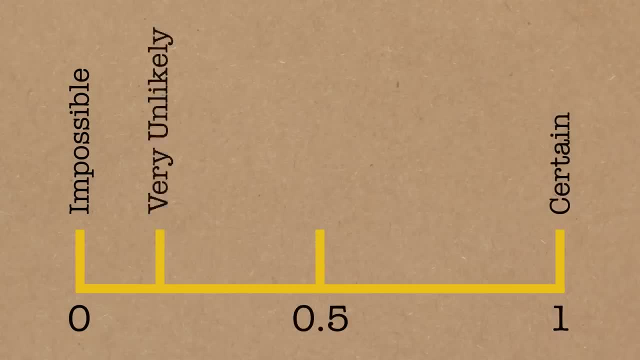 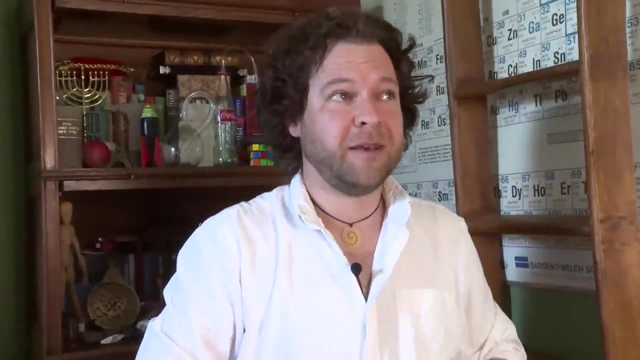 A 50-50 is there. Let's call this very unlikely, unlikely, likely, very likely. I think you get the idea. So that's your scale to use. and here comes the question: What are the chances that there are two people in London with the same number of hairs on their head? 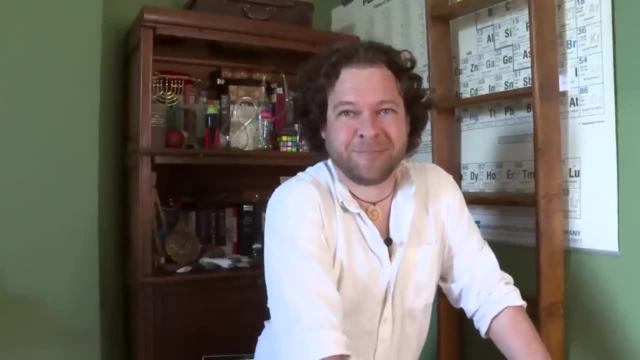 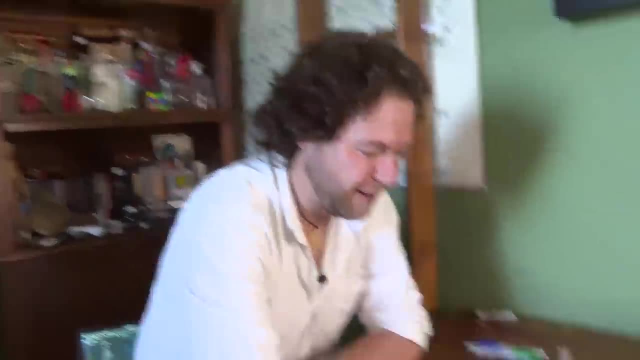 Remember you don't need to give me a number. I want somewhere on the scale Very close to zero. OK, so I'm going to put a Brady, a BH, like down here. Is that fair? Yeah, You want to be closer to zero than that. 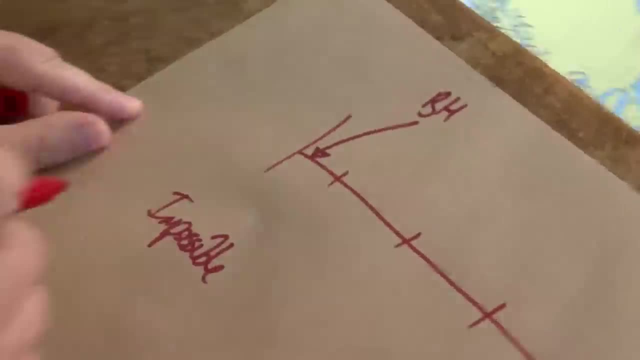 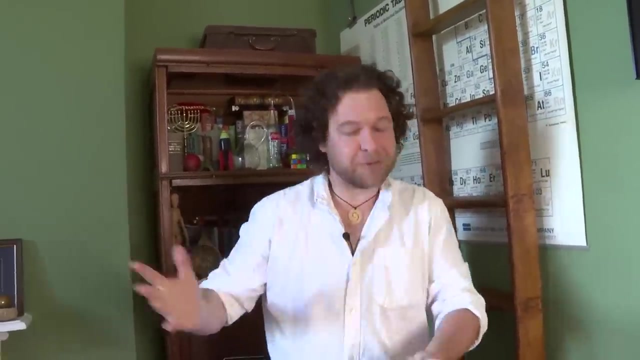 I'd maybe go even a shade closer, but that'll do for now. We're talking ballparks only, but the idea of actually giving me a percentage answer seems nonsense as well, I think So. my claim is- which I will try and answer in the remainder of the video- is that I know exactly where on the scale the answer is. 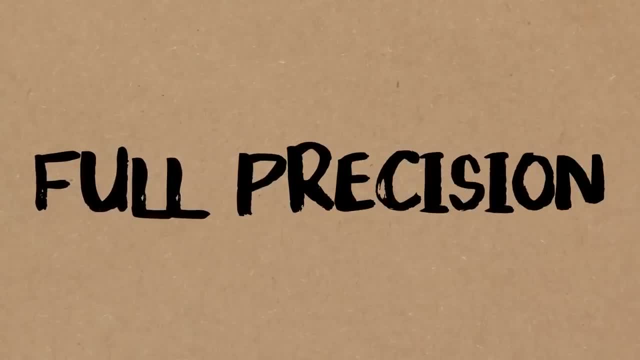 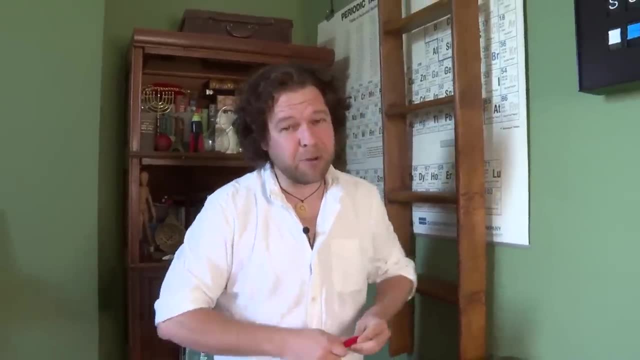 and I know it to full precision. Full precision Like I can nail the absolute full decimal expansion if you wanted me to, And I'm just checking. the viewers have got your gut reactions. You may disagree with Brady. you may agree. maybe you disagree by like a fraction of a percent, Who knows? 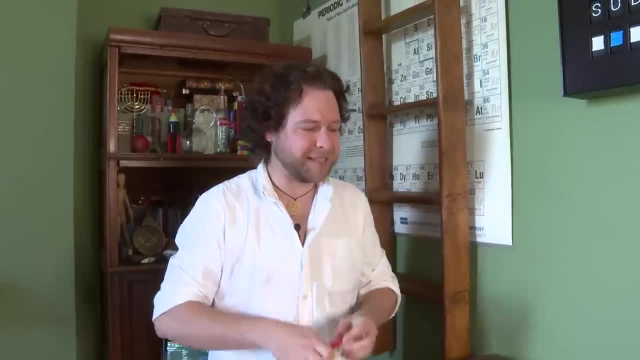 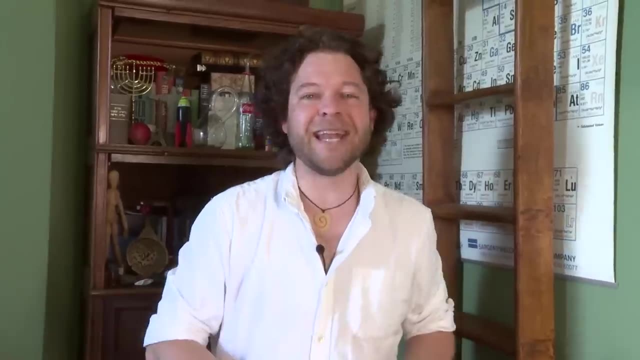 So, er, The reason I'm asking this question is that there's a little bit of background. I want to explain. In the UK there's a qualification you can take post-16. If you're not doing an A-level in maths, you can do something called Core Maths. now 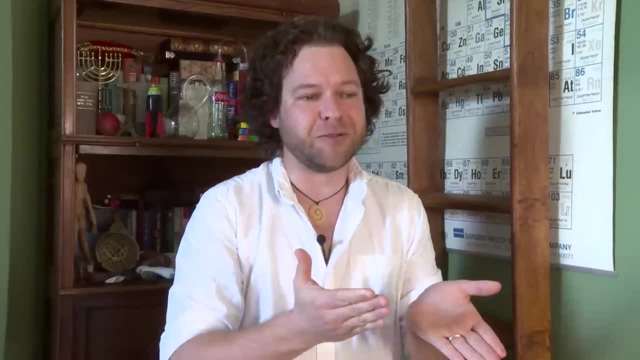 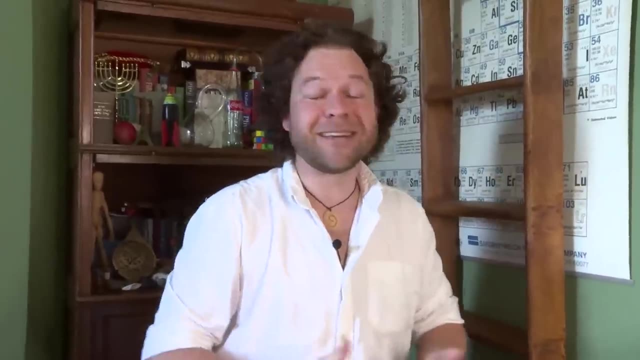 It's a relatively recent thing. It's the maths of everyday life and it's really useful for students to take who are not going to do an A-level in maths but still want to keep some basic numeracy. understand headlines- It sounds like a sales pitch a little bit because I think more people should do it, but the point is part of that course is estimation skills. 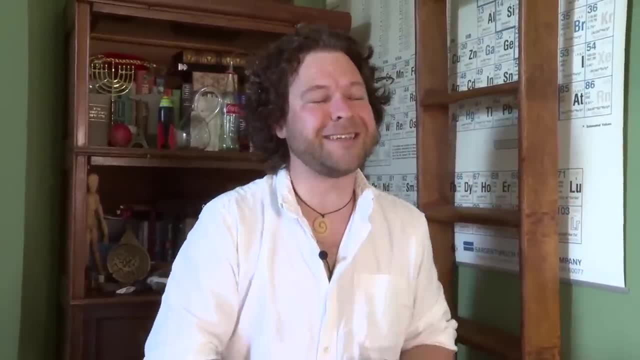 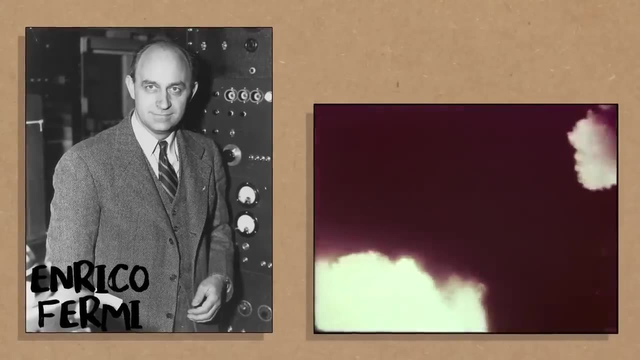 Like, you get examined how well you can estimate, And there's these classic types of questions called Fermi questions or Fermi estimations, where the story is that Enrico Fermi, the physicist, estimated the size of an atomic blast. 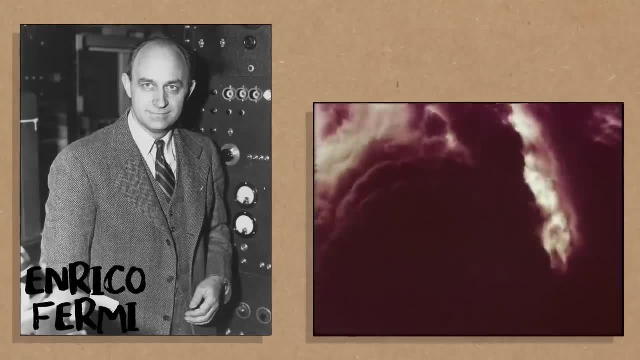 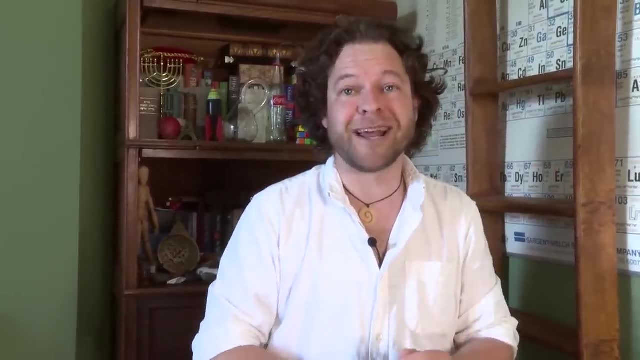 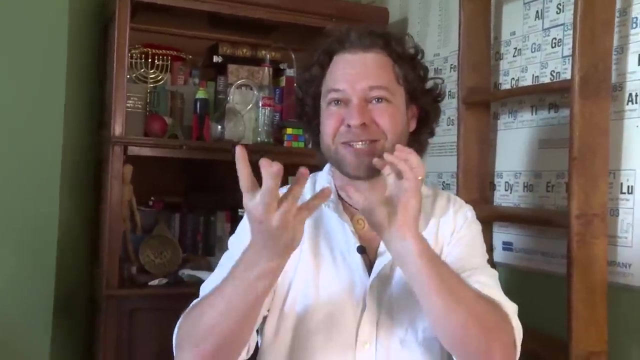 He didn't have any other way of measuring it, so he dropped a piece of paper, noticed how far the blast wind blew it and got the size of the blast within a factor of two. Detail didn't matter, but the size estimate was a really useful skill, and actually knowing roughly how many things occur, er, maybe, I don't know, like the number of people in London, or maybe the hairs on your head- those questions are tied up with this. 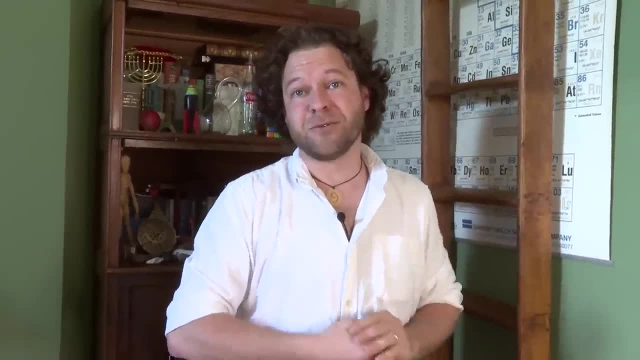 So we're going to use a bit of Fermi estimation skills To solve this once and for all. It wasn't a trick question. you're not counting people with zero hairs on their head, are you? Well, if we did, what's your answer? 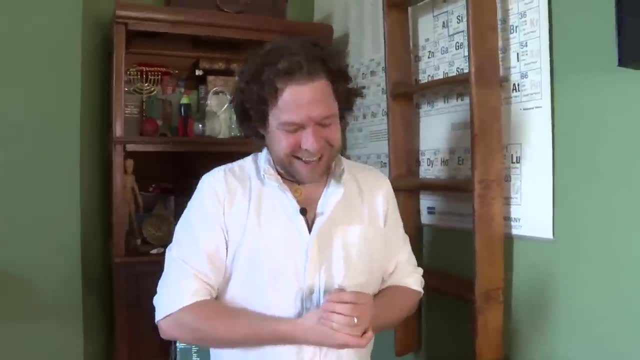 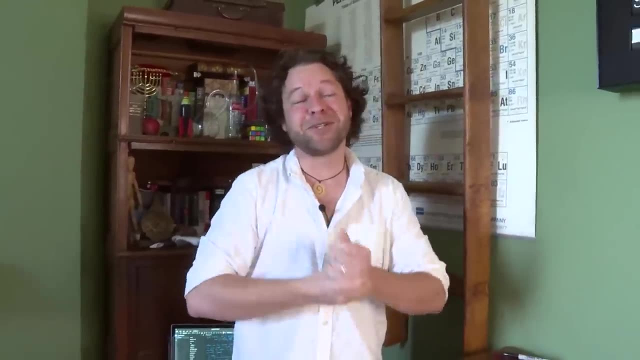 Well then it's one, because there are two people with zero. but I'm not counting that. Brady, inexplicably, that's at the other end of the scale from your guess. But let's say, to be fair to you, that we are not counting that and maybe we should rephrase the question. 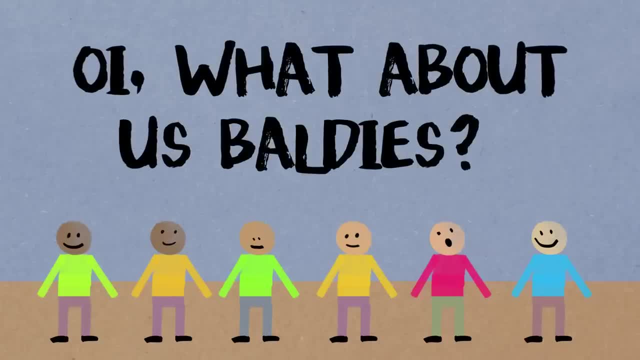 Most people are shouting at the screen, probably thinking: what about bald people? So if we said, what are the chances of two hairy people for whatever, that means having the same number of hair follicles on their head, whatever. 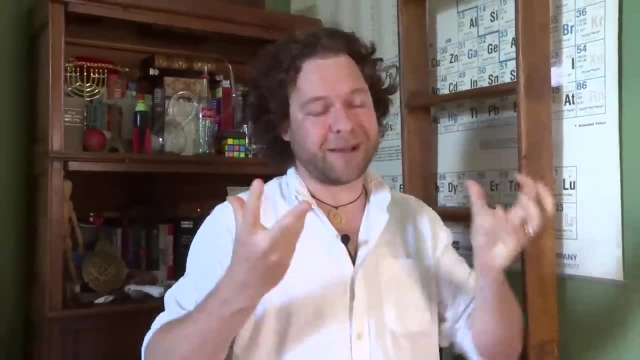 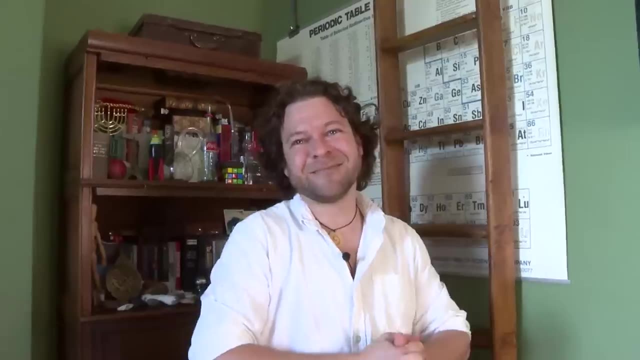 we're going to do some estimation in typical core maths style. How many hairs are on our heads Like? are we talking 10 million? Are we talking 10?? I'm regretting my decision now. There aren't that many hairs on our head. 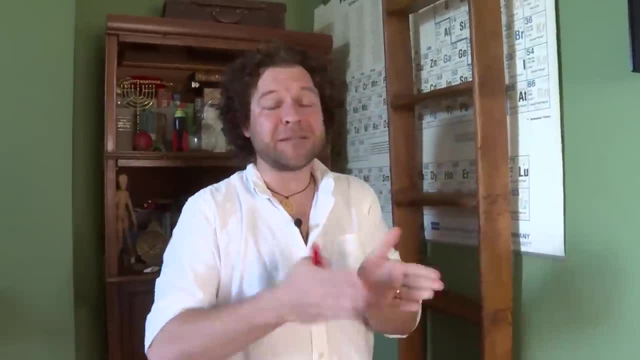 Well, I had a thought about how to give people advice. Estimating stuff is hard, which is, incidentally, why they use these sort of questions as interview questions quite often, Like how many tennis balls can you fit on a jumbo jet? 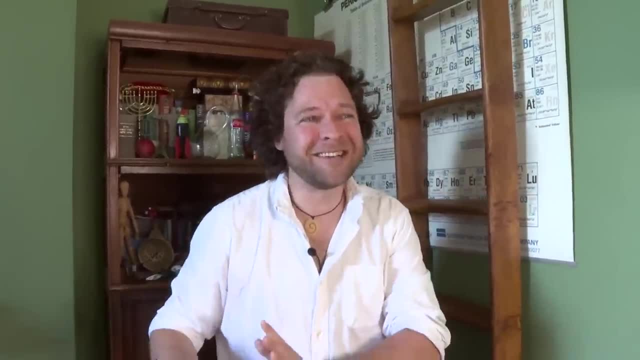 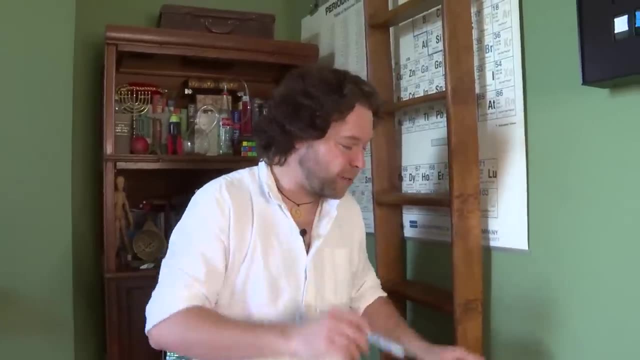 I've heard there's a Google interview question. No one cares about the answer. They care about how you think about it, So Maybe you come up with your own way of thinking about hairs on your head. I had an idea, which is: 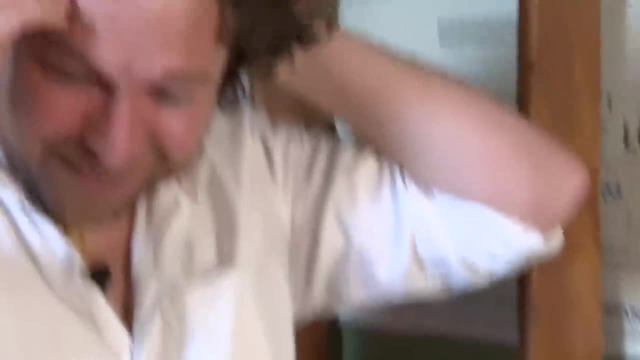 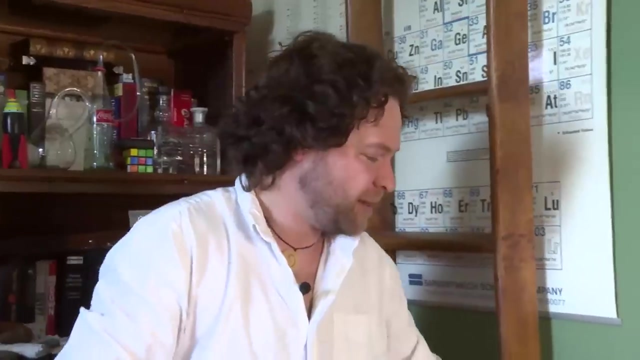 I had a 30cm ruler in my drawer, A nice bendy one, And I can sort of like: Well it's roughly. My hair is roughly like 30cm by 30cm. I mean, I know my hair is a source of contention among Numberphile viewers. 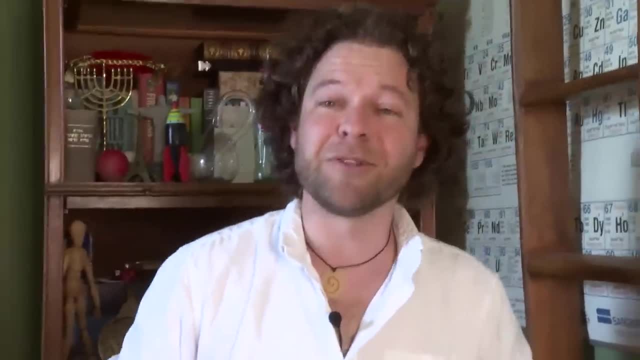 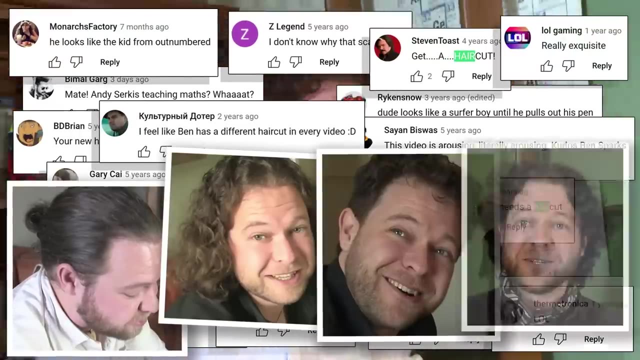 There's been incidences on camera where I had questionable hair, And possibly still do. But well, leaving that aside, You think I haven't just put them on screen? That's cute. I talked myself into that, didn't I? 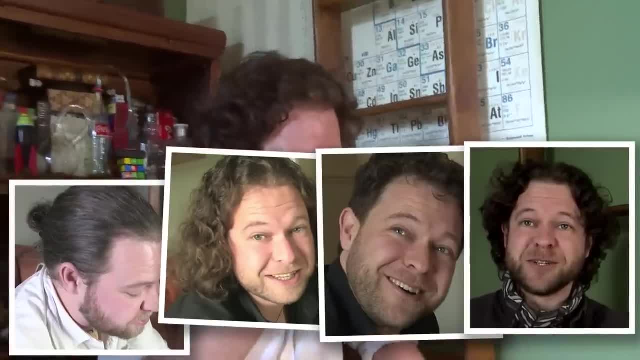 New Numberphile video, new haircut: That's my motto And I think actually, if you drill down, The size of my head is kind of within grasp of centimetres And if you think about like a 1cm squared patch, 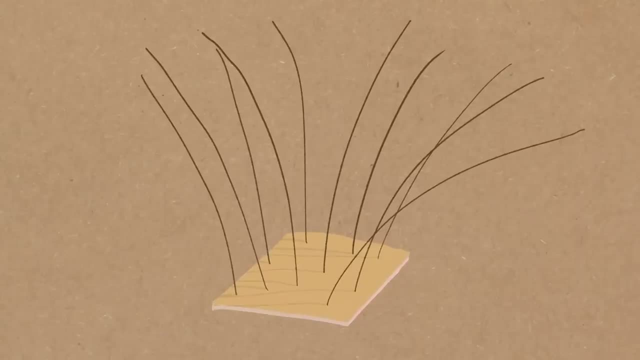 No close-ups. alright, I think we can get an order of magnitude. So I think there's probably more than 10 hairs in a centimetre squared, Like it feels like sparse- Probably not as many as 1,000.. 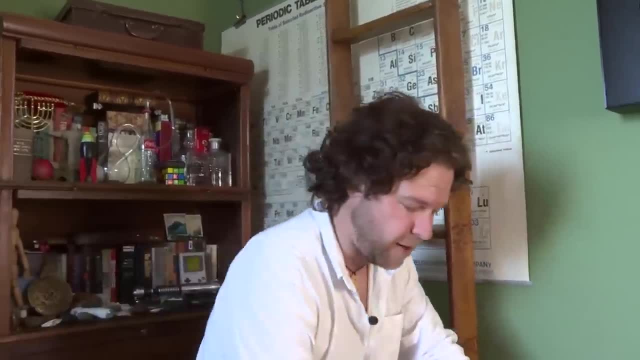 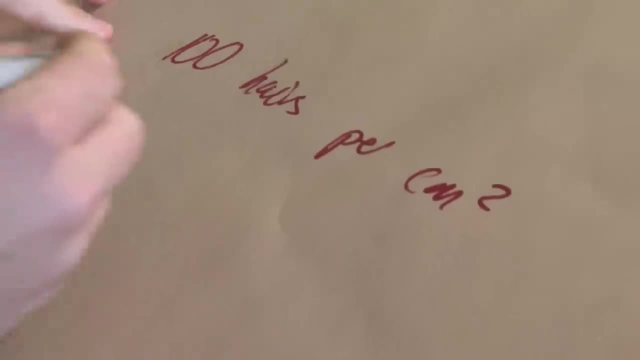 So let's pick 100.. I'm gonna start writing some stuff down: 100 hairs per centimetre squared, And then, roughly, let's get the size of my head. So I mean I've already waved the ruler around. There's 30cm by 30cm, Approximately 900cm squared times 100.. 90,000 hairs. How do you feel about that? Loads of people in London have the same number of hairs on their head. You wanted to change your answer. 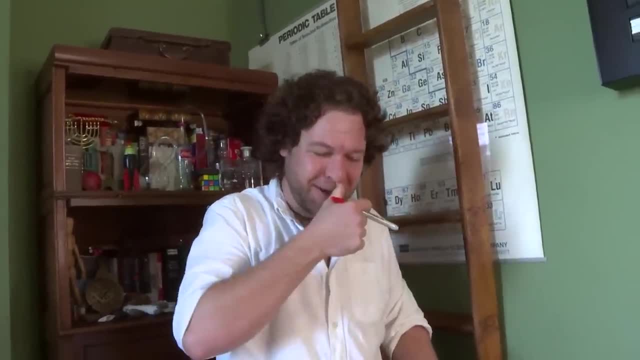 I'm glad we are already acknowledging that there is doubt creeping into your earlier gut reactions. So let's just settle it once and for all. I don't even trust my estimation, But if we went to, let's call it, 100,000,. I don't think many people are gonna be an order of magnitude out from that. Incidentally, I did do some research on this and apparently red-haired people have fewer hairs. Quality, not quantity, apparently, is the name, But roughly people are estimating between 50,000 and 150,000.. 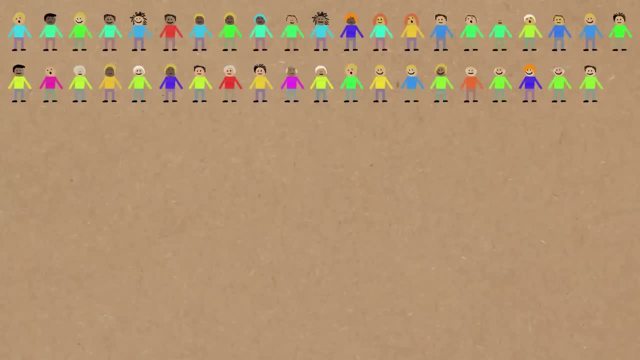 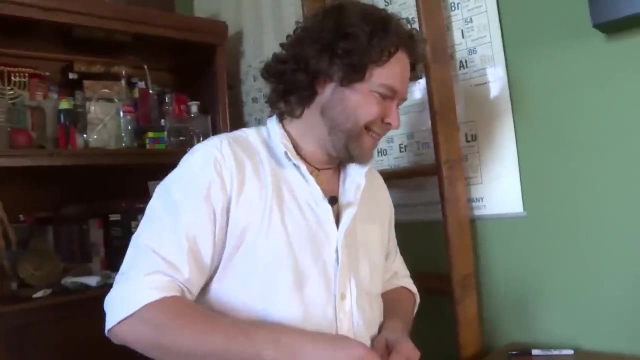 So I'm really glad our estimate is pretty good. How many people in London, Brady, What is it? Is it like 12 million Or 8 million? And anyone who was shouting at the screen earlier when I asked the question would be like: it depends what you define as London, right, Greater London, The City of London. However you really do it, I think we're in millions, Agreed. Yeah, Like, even if you go small And let's say Greater London. I reckon about 8 million. 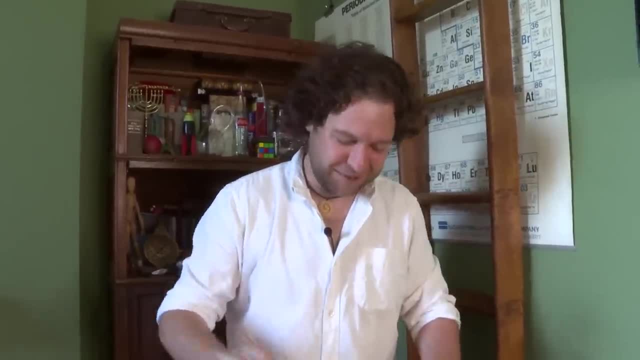 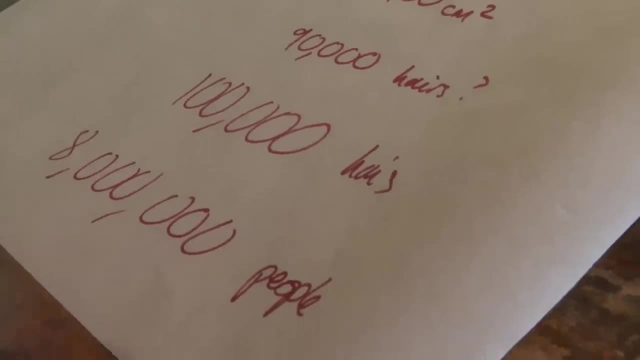 But again, I don't actually care, because I'm just gonna say 8 million. You'll see that the actual detail doesn't really matter. Now you've already upgraded your estimate, But let's think about why I'm gonna do what they call in the trade a piece of common sense. 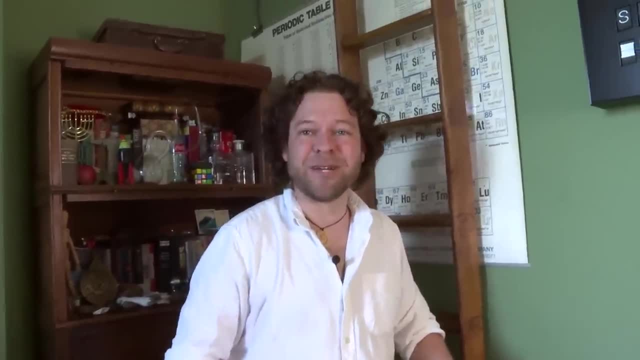 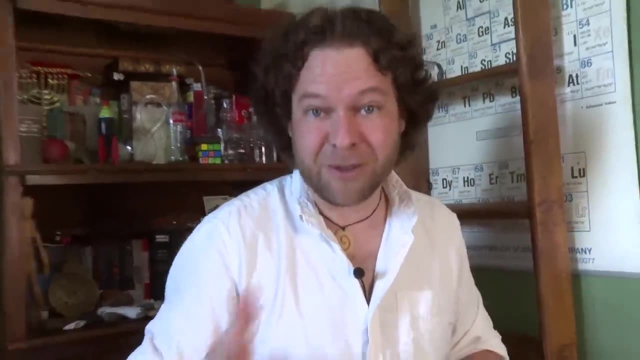 Which is the name for a mathematical theorem which everyone thinks is really profound and everyone else is like, well, that's just obvious. But this is called the pigeonhole principle, and if you have heard of it, well done, You might think it's common sense. 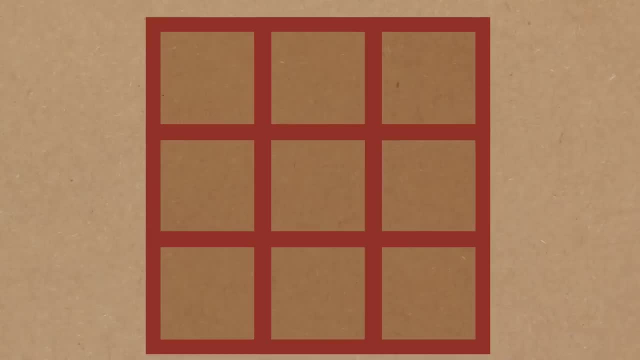 If you haven't heard of it, it's time you heard of it. So if there are nine pigeonholes in this little grid here and I had eight pigeons, they could arrange themselves all through and there'd be a gap. 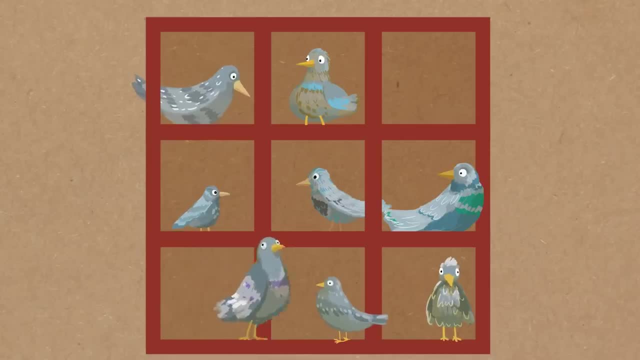 They've got one pigeonhole each, They could arrange themselves to double up. There's no rules against it if they're particularly cosy, But they don't have to. My point is, if I have nine pigeons, they could have a pigeonhole each. 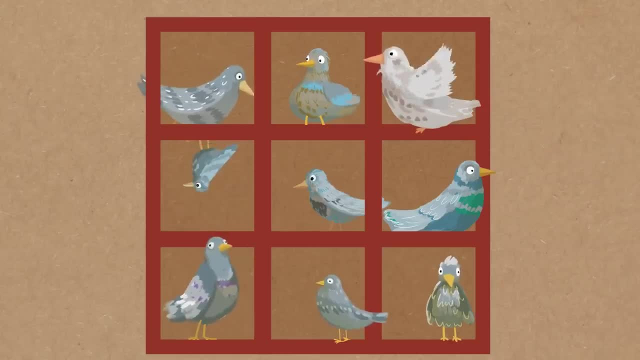 They might double up, but they don't have to, Whereas if I have ten pigeons, two pigeons are sharing. At least This is known as common sense to most people, and other people call it the pigeonhole principle, and it's a surprisingly profound useful result in very different situations. 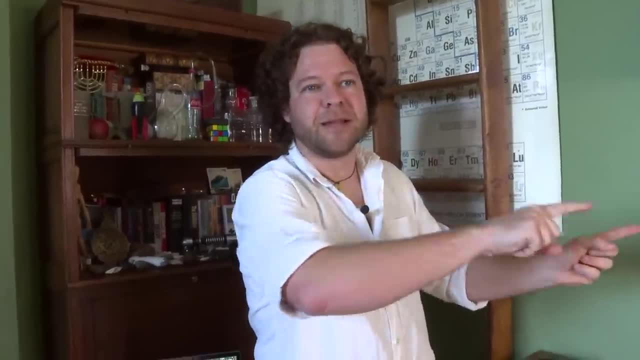 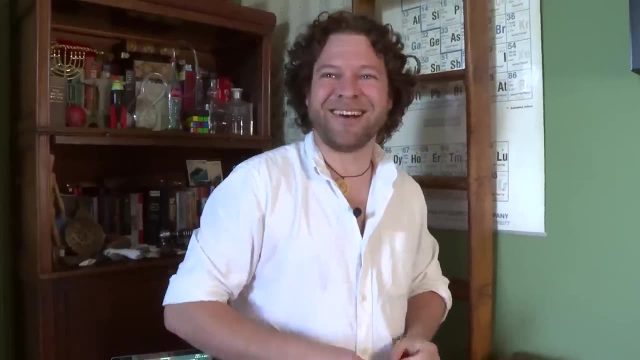 If you've got more things than options, then the people choosing options are going to double up And I think by the velocity of your nodding you have seen how this might apply. Let's imagine all the people in London are choosing an amount of hairs. 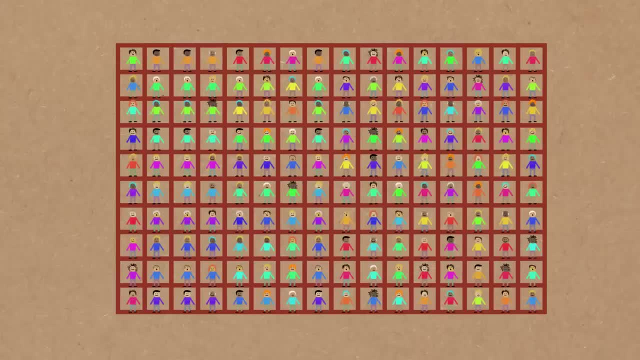 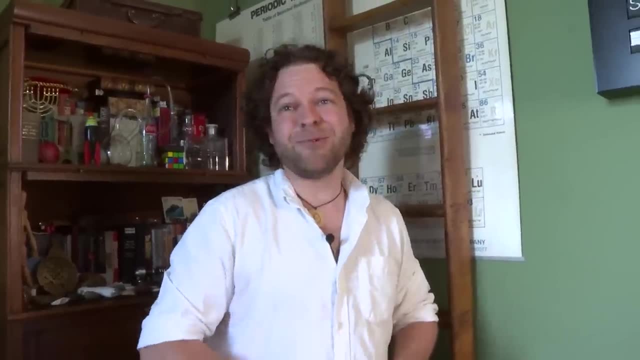 Even if they're making up a number right, They're just: I have 963 hairs and I have 900,000, whatever They want to be unique, They're trying to be, But if eight million people try it, 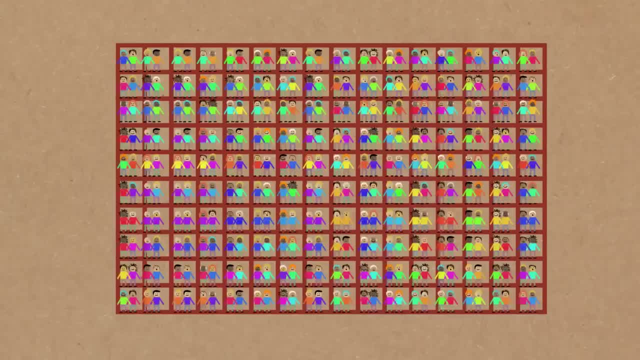 and there's only roughly 100,000, or even 200,000, or even 300,000 options. two of them are going to duplicate. There's nothing we can do about it. I'm sorry to break it to you. 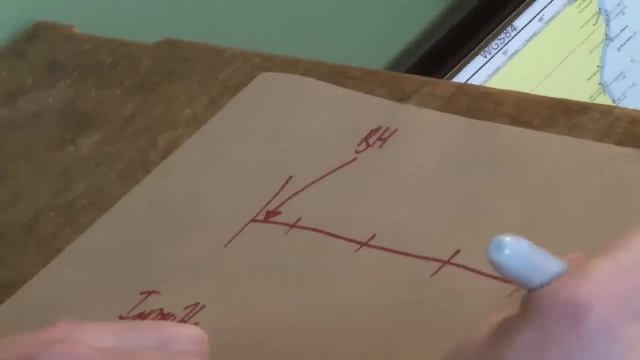 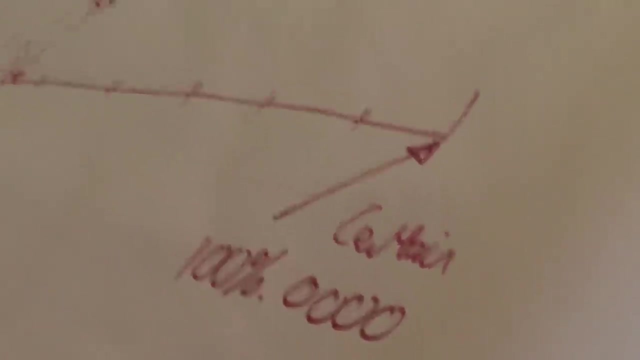 Not only are we not down here, we are precisely there. It's 100%, And I said I'd do the full decimal expansion if you want it, but it gets pretty dull pretty quickly. So I like this question because it feels like our gut reaction. 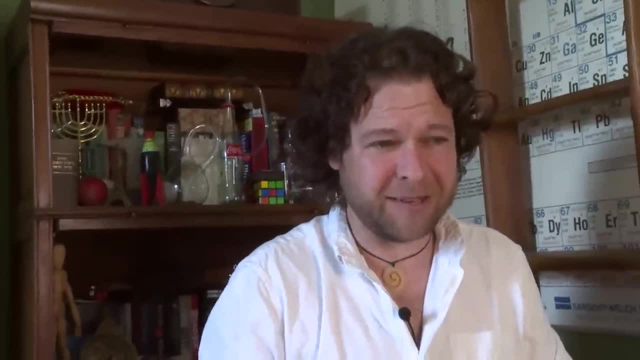 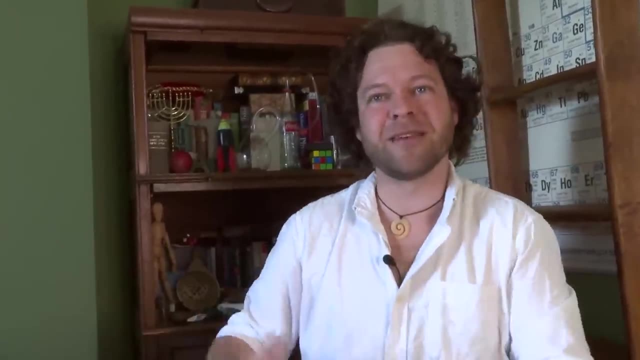 goes wrong quickly, And I think it's because we're not very good at estimating without training, Incidentally, why core maths is a good thing to study And it's nice to actually do an exam where you're rewarded in this common sense way of thinking. 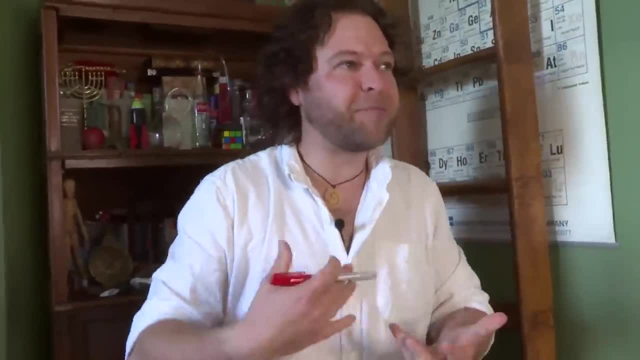 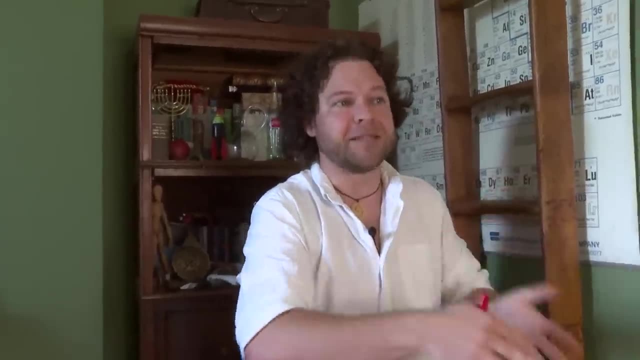 I studied maths, Ben, and I got it wrong terribly. I think math petitions particularly you've done your share of maths, maybe more than the majority of people in the world are actually less good at the basic common sense estimating than other people. 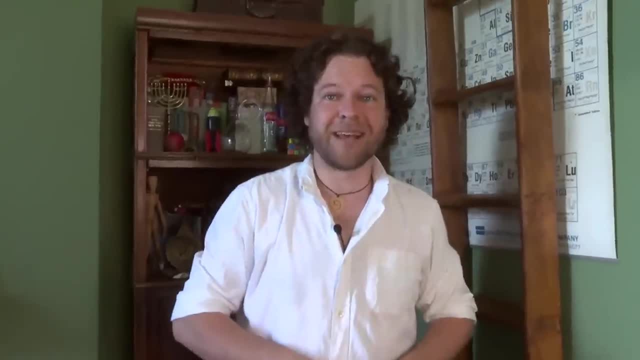 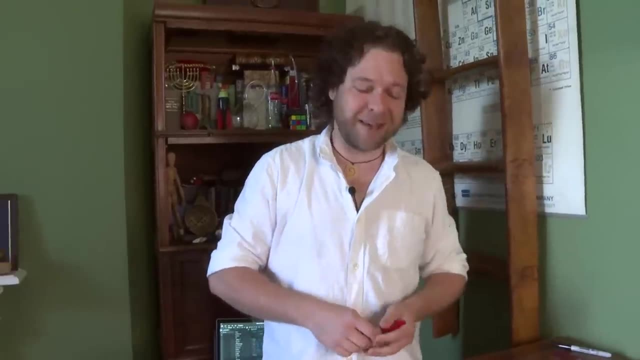 And people who have to do a lot of this every day are better at it. It just takes practice, And studying maths doesn't involve lots of it, which is why this is an interesting qualification to talk about And a good skill to have whatever qualifications you study. 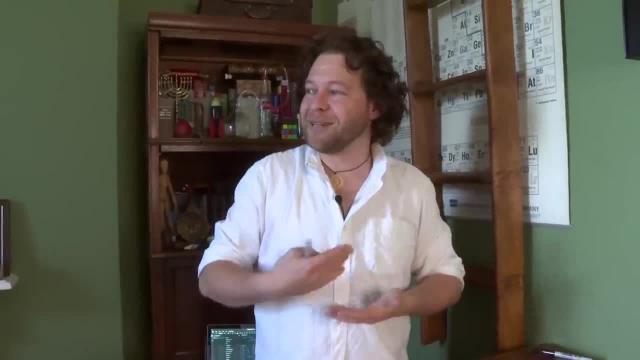 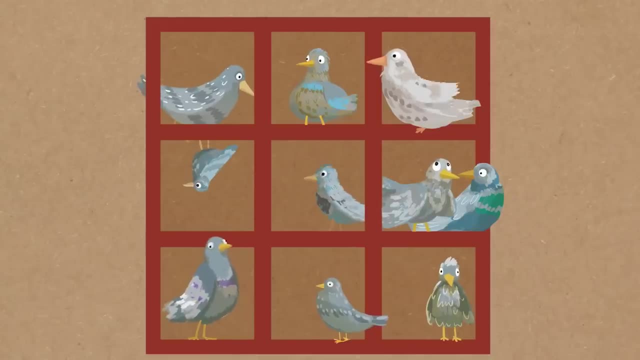 The art of estimation is important, And in this case what's nice is the probability question not only has a definitive answer, all you need is rough ballpark estimates. to nail it down completely, Turns out that the pigeonhole principle has lots of important applications. 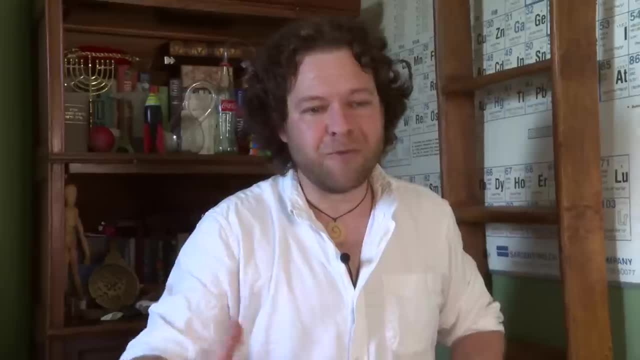 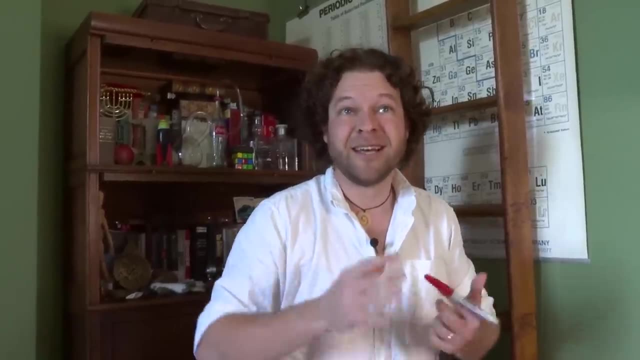 If you want to look at the possibility of things duplicating. if you make up a random password with a certain key space and someone else makes a random Like, what are the chances of duplication occurring? You realise it's the same sort of question and that's important. 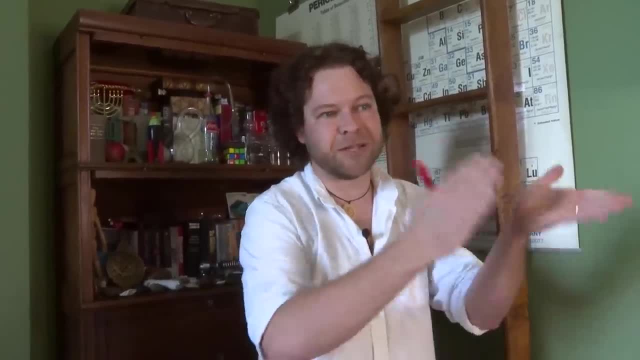 And there are links to another cliche problem called the birthday paradox, Like: what are the chances two people share a birthday? It's not quite the same, but if you have enough people in that question, if you have 366 people in a room,